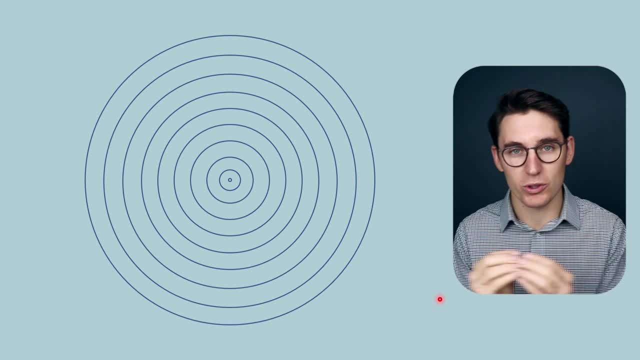 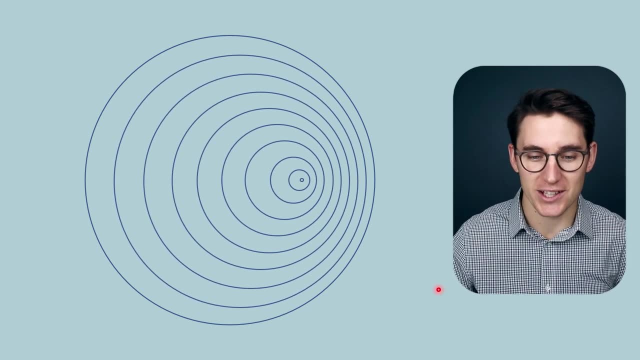 remains the same. Now, if that source of sound was to move, we will get a change in the frequency of that wave. As that sound source moves, the frequency of that wave will change. We can see that the direction in which it's moving. we get an increase in wave frequency. 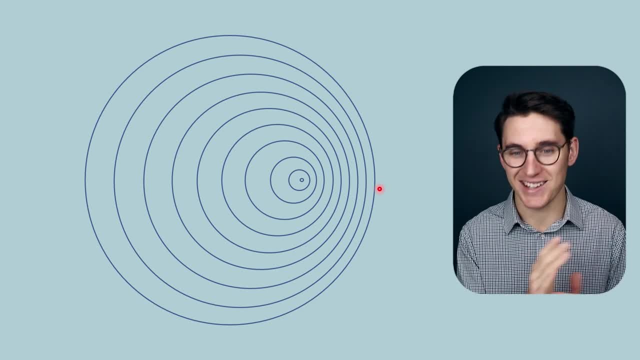 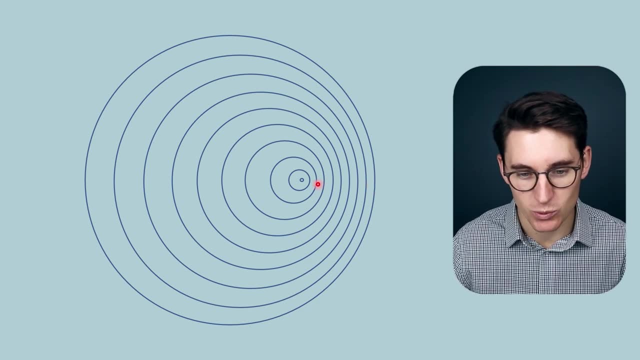 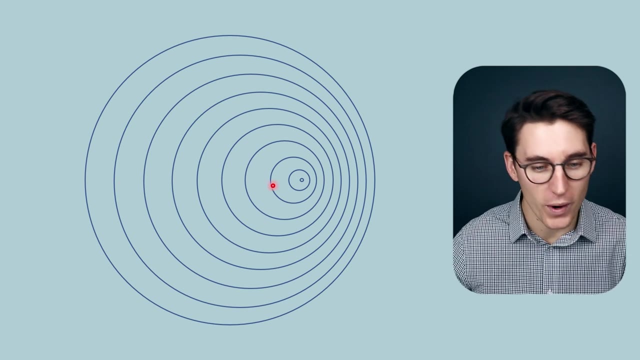 The number of waves passing a particular point per second increases, The pitch of our wave will increase. As that frequency increases, our wavelength as well as our period decrease. Now the opposite is also true. Where the sound source is moving away from the wavelength gets. 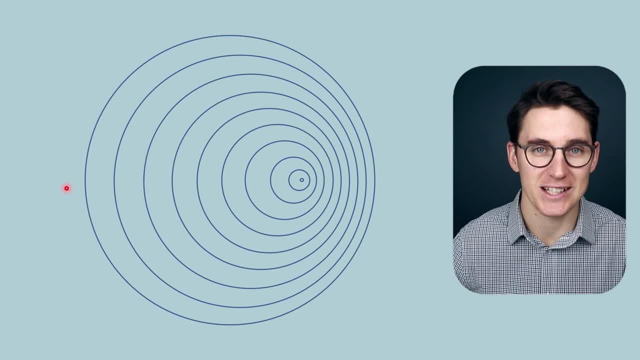 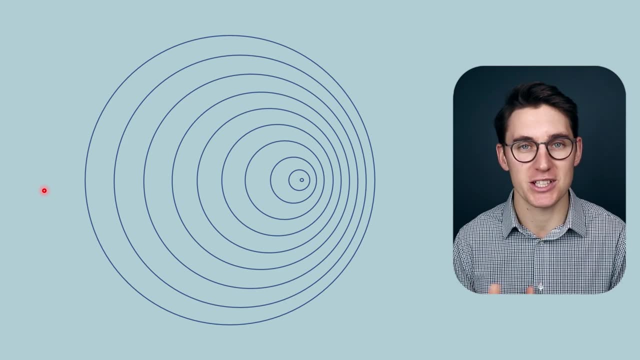 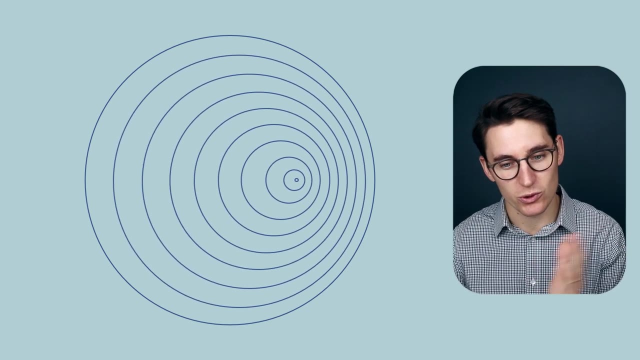 longer, our period gets longer and our frequency decreases. Our pitch of this wave decreases. So it's the movement of that wave that changes the frequency of the wave. Now we can see that the difference between this original frequency and the frequency once that sound source moves is what's known as the Doppler shift. Now we have a source. 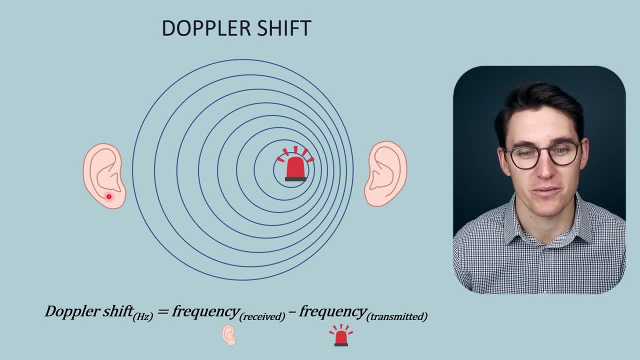 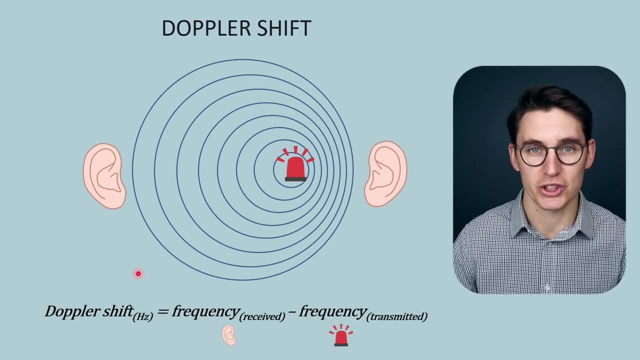 of the sound wave as well as receivers of the sound wave. Now it's this observed change in frequency that is known as our Doppler shift. And to calculate the Doppler shift, which is a change in frequency, and we measure that in hertz- is the frequency that we receive this change: frequency minus. 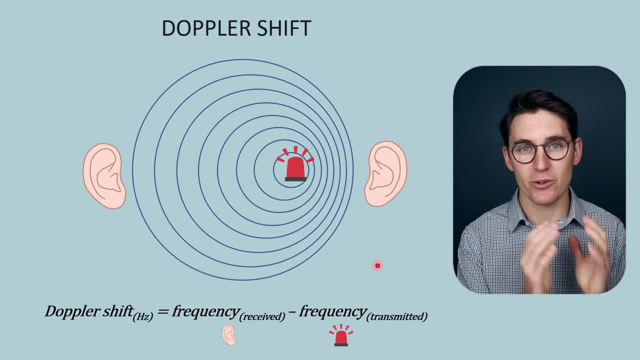 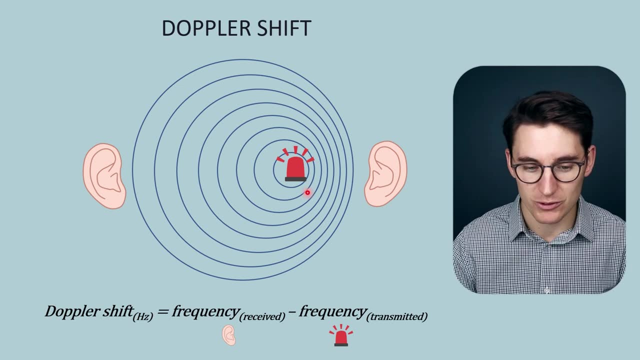 the transmitted frequency from our source. So what was the original frequency? What is the new frequency? The difference between those two is what's known as our Doppler shift. Now, our Doppler shift here will be a positive value. Our frequency received is higher than. 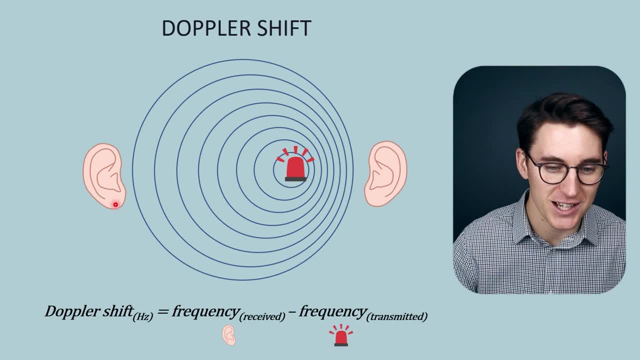 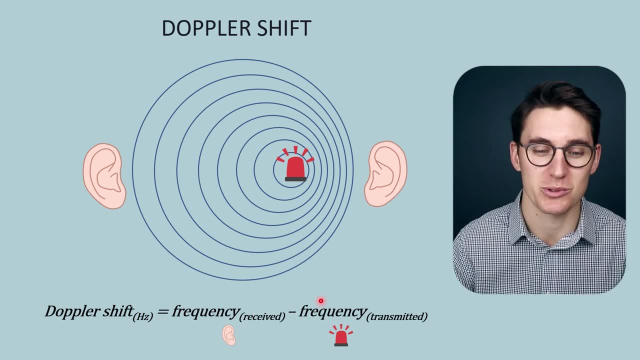 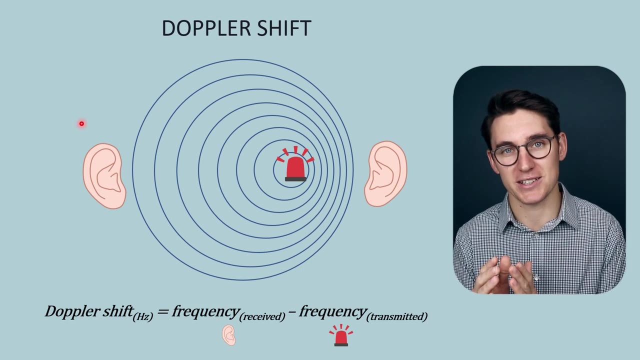 our frequency transmitted. The Doppler shift on the other side here will be a negative value. We will have a negative Doppler shift. Our original frequency, our transmitted frequency, is higher than the frequency that is being received on this side. So the Doppler shift is a result of the Doppler effect. Now in 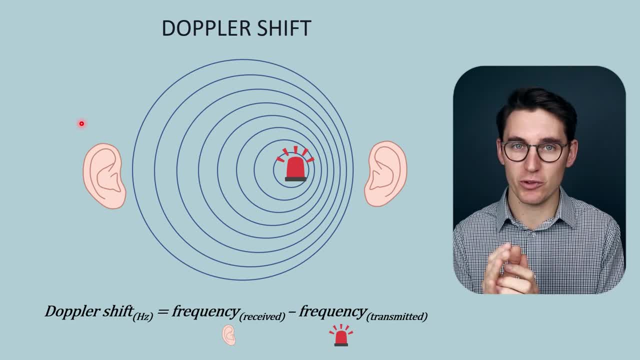 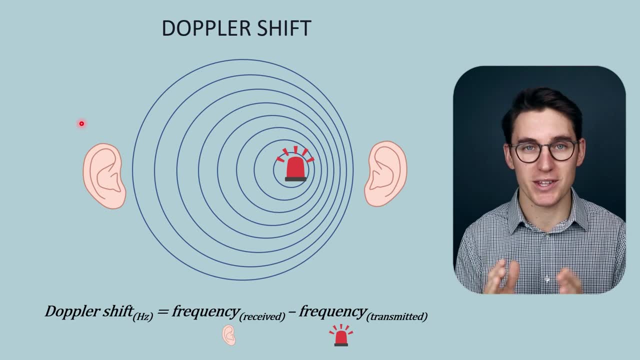 order for Doppler shift to occur. either the source of our sound is moving, the receiver or the receptor for that sound is moving, or there is a reflector of that sound that is moving within the ultrasound field. Now we can use this phenomenon in ultrasound when. 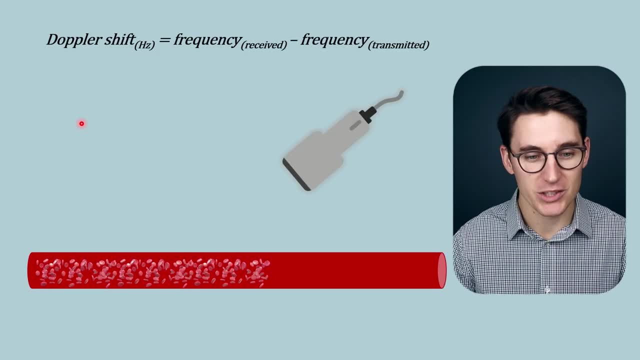 trying to measure the speed of something within our ultrasound field. So if we take this in this example, here we have our ultrasound machine and we have blood within a vessel that is moving at a specific velocity. Now, if that blood is moving towards the ultrasound, 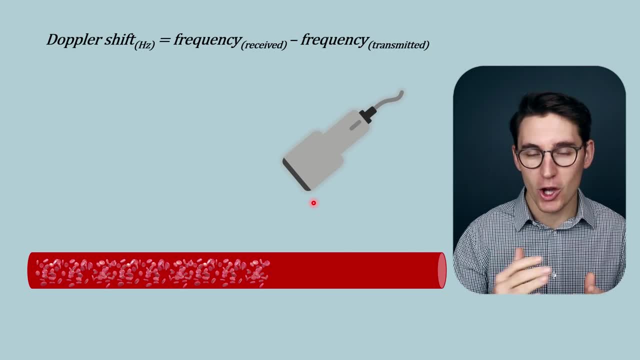 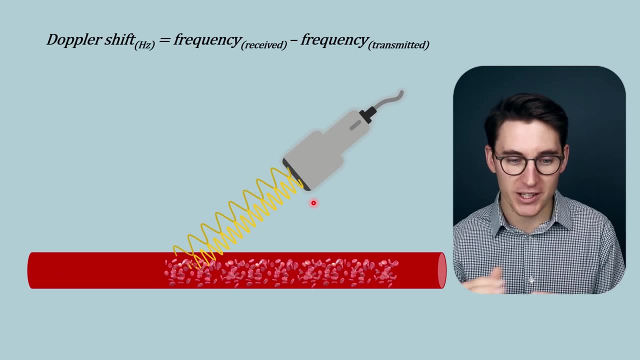 machine. ultrasound pulses that are incident on that blood will return back to the ultrasound machine at a higher frequency. So let's have a look at what that looks like here. Blood is moving towards the machine, the reflected ultrasound pulse, the echo, coming back has. 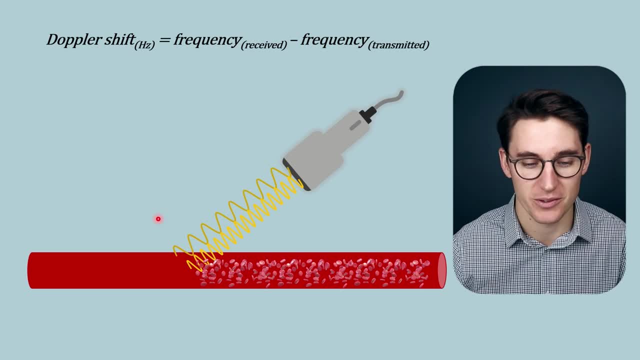 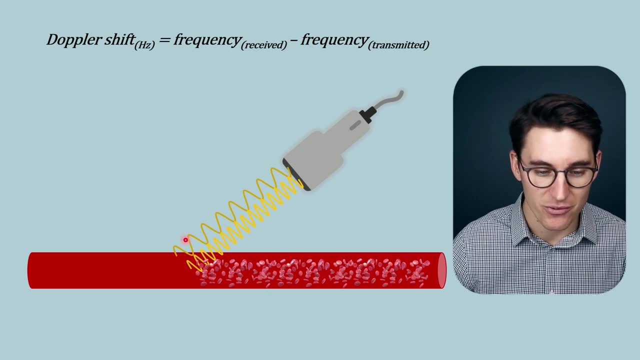 a higher frequency, We have a positive Doppler shift. Now this change in frequency, this Doppler shift, is proportional to the velocity of that blood And the value that we get back here is a scalar value. it has magnitude but no direction. And that value we get back here. 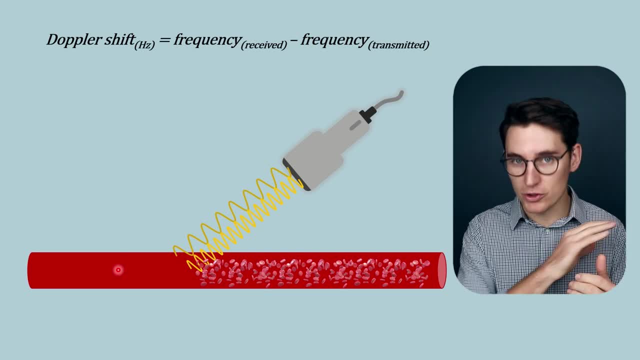 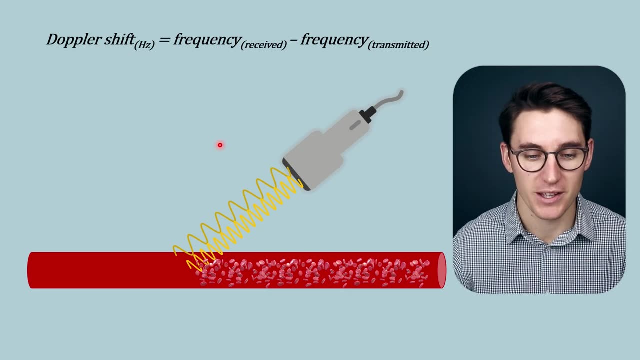 is a speed value that we can calculate. Now, as that blood moves faster and faster, the change in frequency will become greater. We get a higher and higher frequency returning echo. Now the opposite is also true If that blood was moving away from our ultrasound. 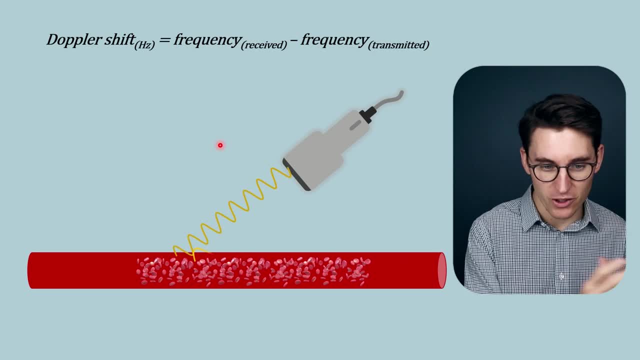 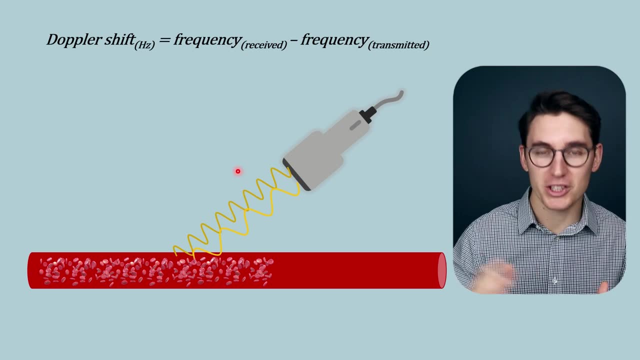 transducer, we would get a negative Doppler shift shift, the frequency of that ultrasound wave returning to our ultrasound machine will be less than the original frequency. here Now I've mentioned the Doppler shift is proportional to the velocity of that blood. but we have 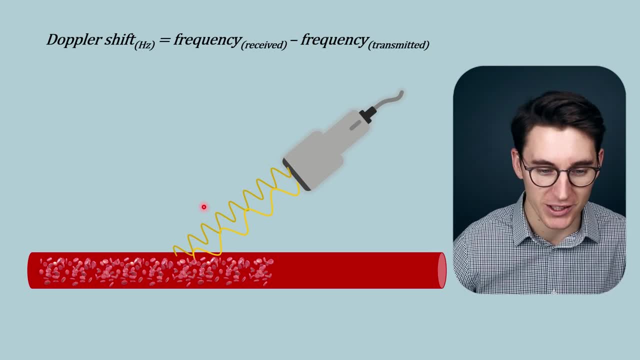 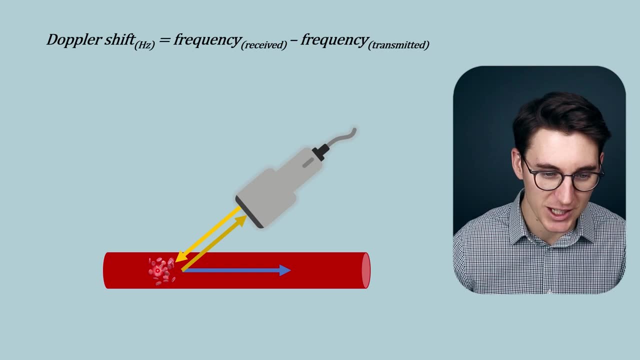 no directional component here, we only have magnitude, that we are measuring the magnitude of Doppler shift, And we need to break these down into separate components because our ultrasound frequency, coming in towards the moving object, is at an angle of incination to the movement of 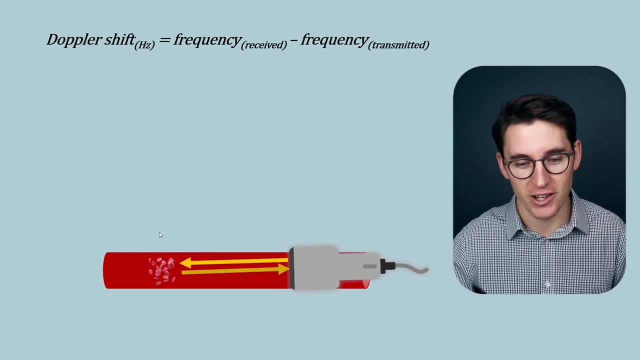 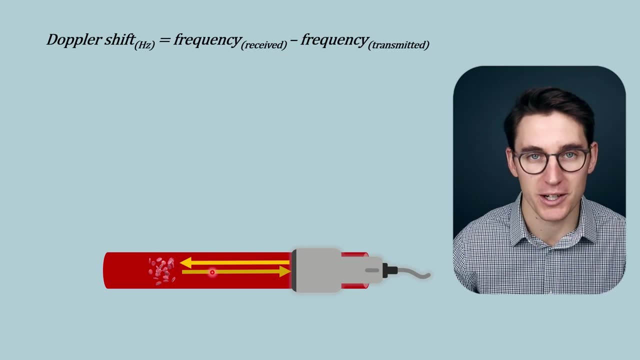 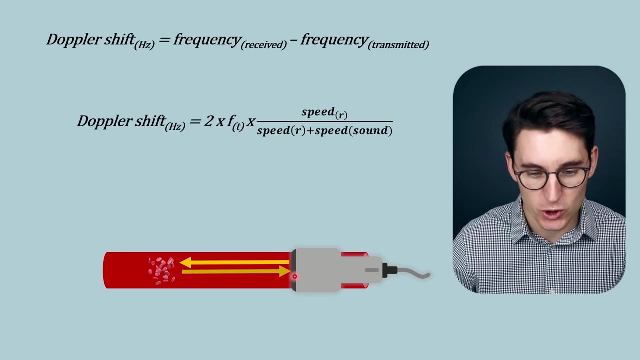 that object. Now, if we were to get rid of that angle, have our ultrasound machine directly in line with the movement of blood here? we can then calculate the speed of the blood moving here, because it's directly proportional to that Doppler shift. We can use an equation: the Doppler shift is two times the frequency of our transmitted. 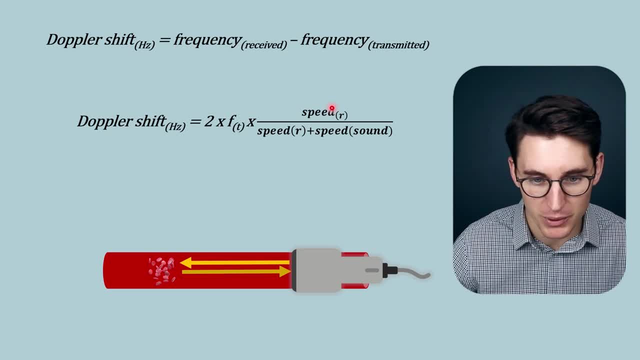 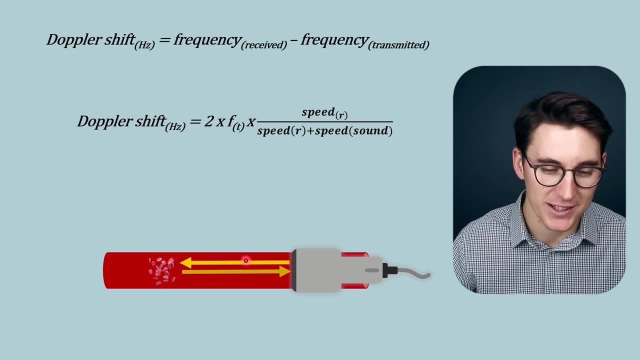 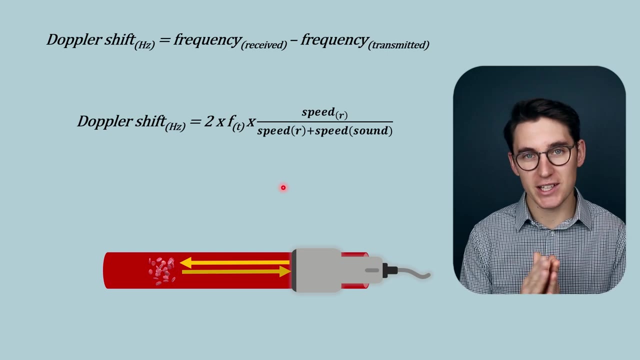 ultrasound pulse times by the speed of the blood moving towards the ultrasound machine over the sum of both the speed of the blood and the speed of sound. Now, when we look at this fraction here, the speed of blood moving in tissues never really gets higher than 200 cm per second. 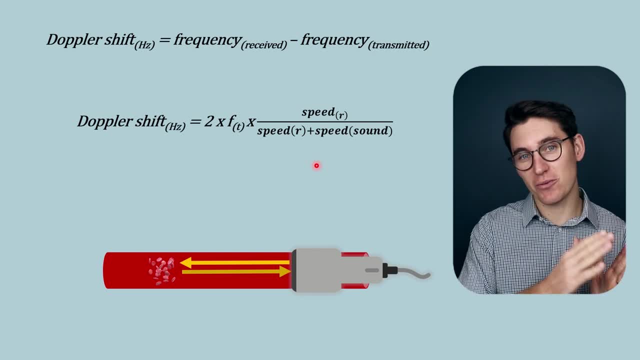 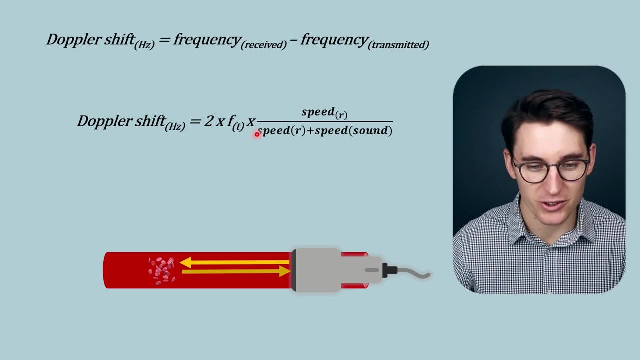 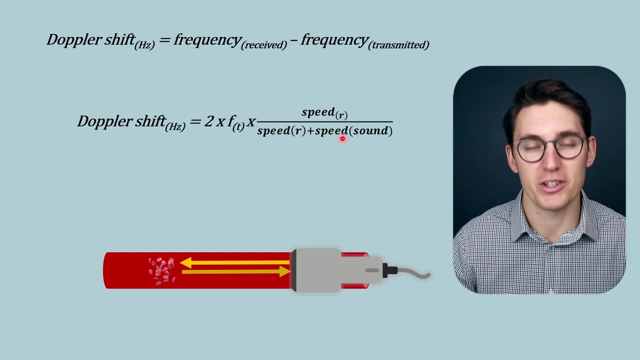 And the speed of sound in cm per second is 154,000 cm per second. We see we are dealing with very different magnitudes here And as a result this speed of the red blood cells in our denominator here is often ignored because it's such a small fraction of the speed of sound of ultrasound within our body. 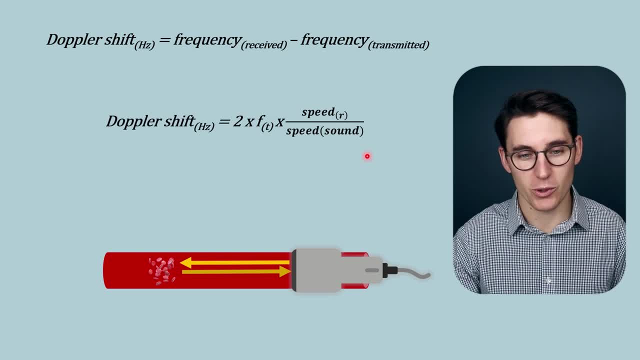 So the speed of blood moving in tissues never really gets higher than 200 cm per second. So often you'll see this equation written like this. Now I'm not going to get into why, but this 2 here is a coefficient within our Doppler. 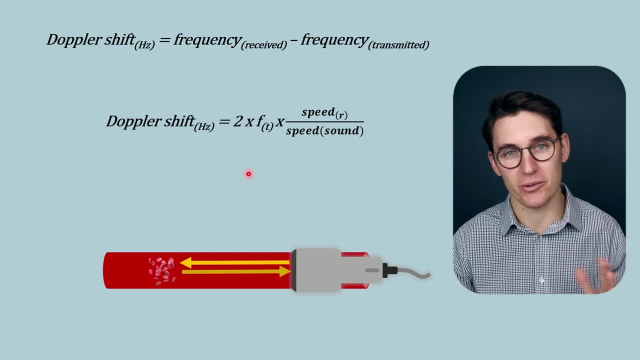 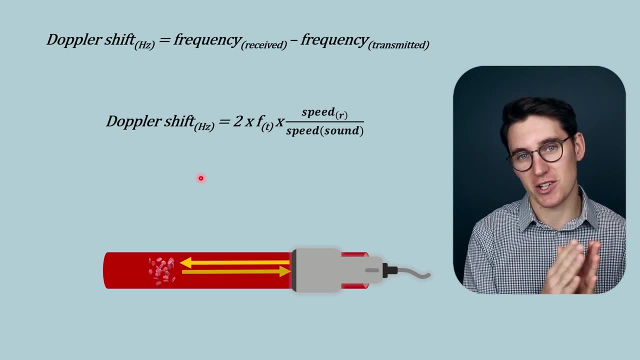 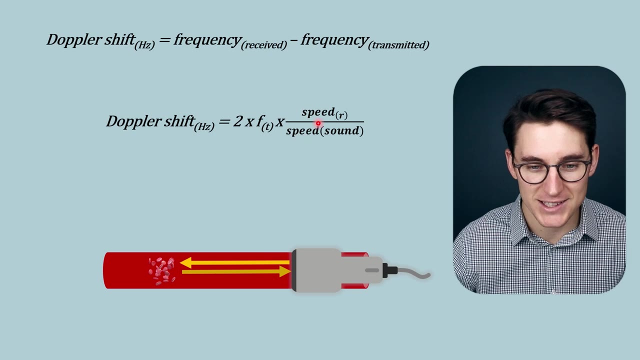 shift equation, And that's needed when we have a moving reflector. It's got to do with the speed of sound, of both our incident ultrasound wave as well as the speed of the reflector shifting that ultrasound wave in the returning echo. Now here we are, using the speed of the blood moving within the vessel and seeing that. 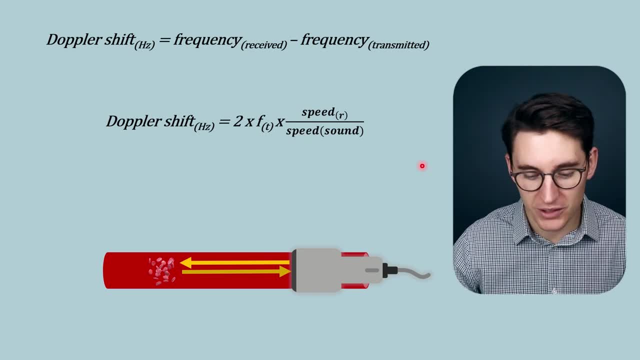 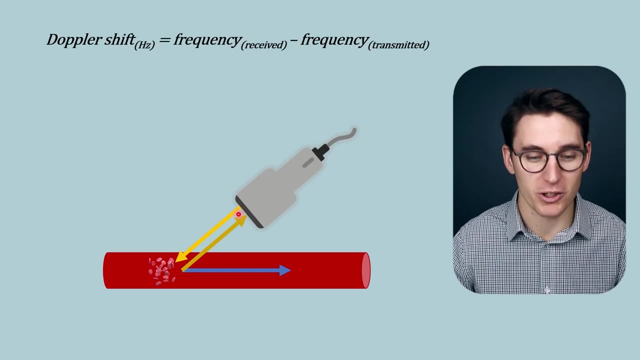 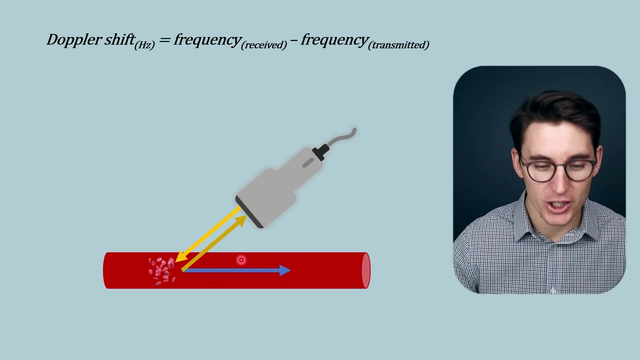 that speed is related to our Doppler shift. In the previous examples, we had an angle to this ultrasound machine. Now, because we can break this system down into multiple different components- the velocity of our blood as well as the Doppler shift- at a specific angle, we can use trigonometry. 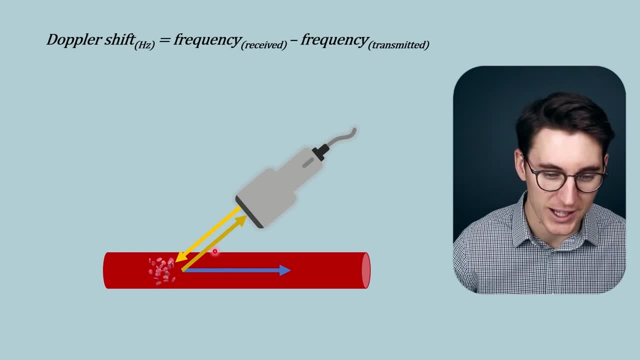 to calculate this velocity value if we know this angle of intonation or our Doppler angle here. Now what we are trying to calculate is the velocity here and what we actually have, the known value, is our Doppler shift. So we can use trigonometry to calculate this velocity value. 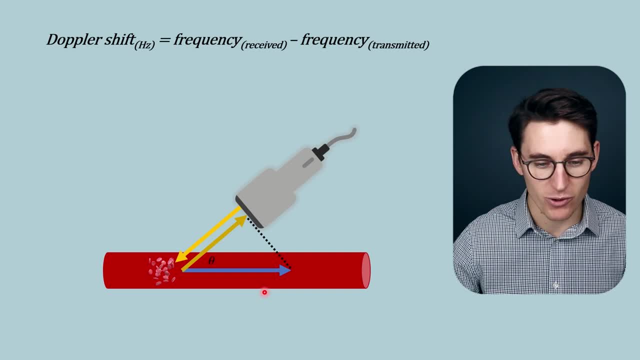 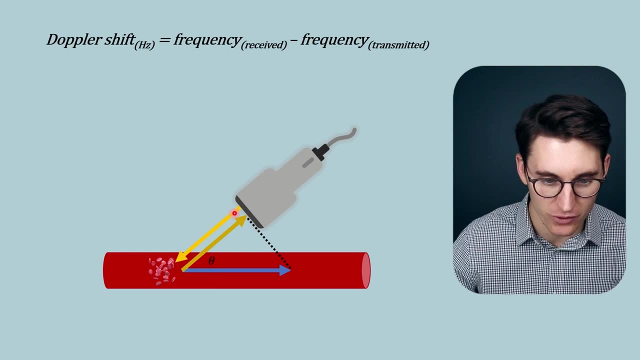 And so we do a Doppler shift heading towards the ultrasound machine. We can create a right-angled triangle here with our Doppler angle. If we take the adjacent side of this right-angled triangle and we're trying to calculate the hypotenuse here, we can use the cosine of this angle to have our adjacent or our Doppler. 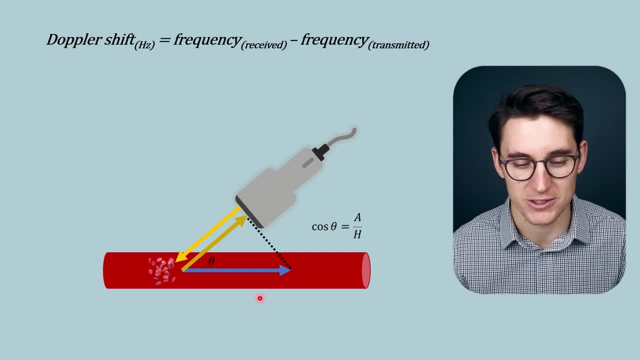 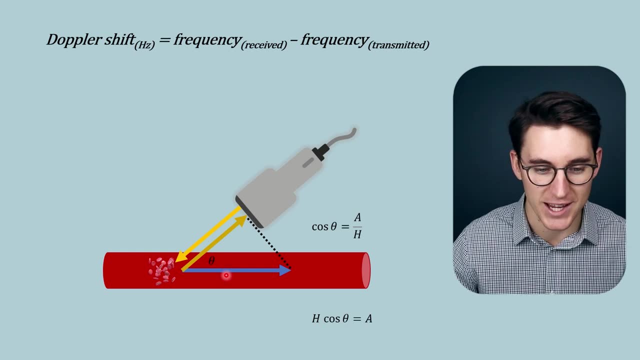 shift over the velocity of the blood travelling through the blood vessel. And if we rearrange that equation, the velocity of blood travelling through the blood vessel times by the cosine of thatCoronautic of this angle, will give us our Doppler shift, or the speed that we had calculated from our 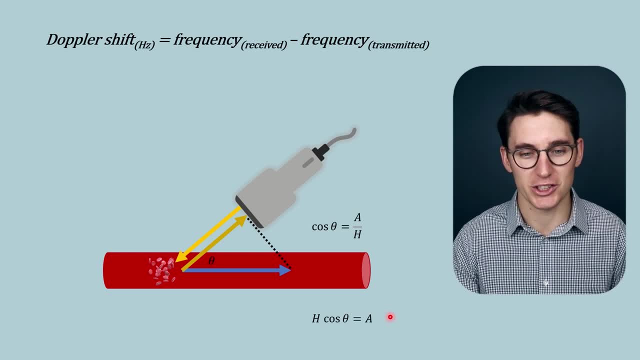 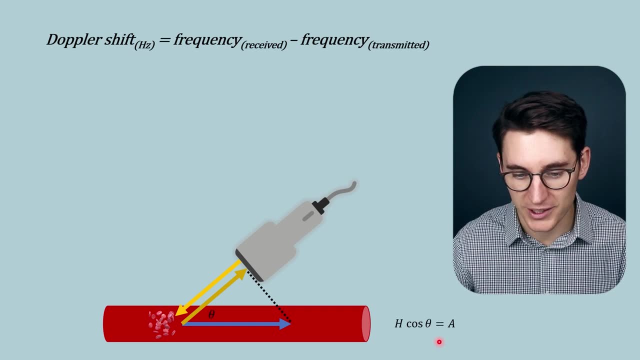 ultrasound machine. Now, when we looked at that initial equation, we had the speed of blood moving through tissue over the speed of sound. Now we can plug in this new formula that we've calculated here, which compensates for an angle of intonation, to get what's known as our Doppler equation. 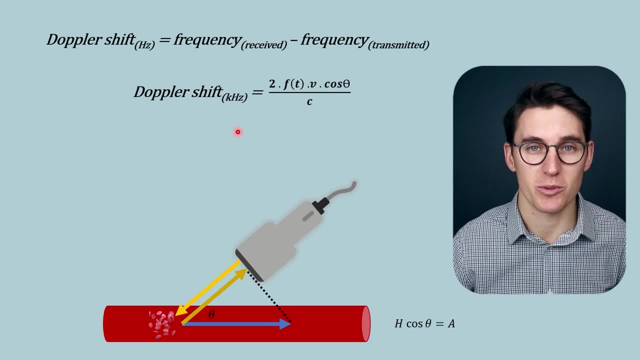 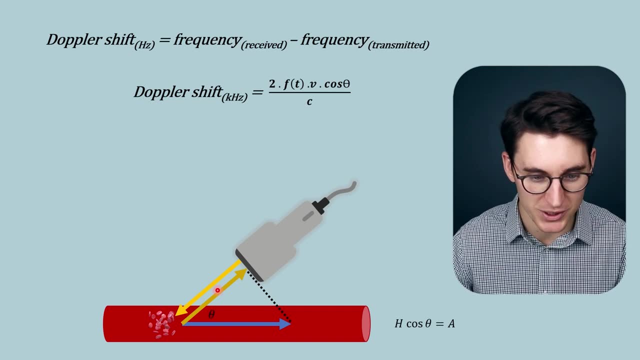 Now we can see here that the Doppler equation and the Doppler shift equation that we calculated in our previous slide are essentially the same. Our Doppler shift is two times the frequency of our transmitted ultrasound pulse times by the velocity of the moving component within our ultrasound. 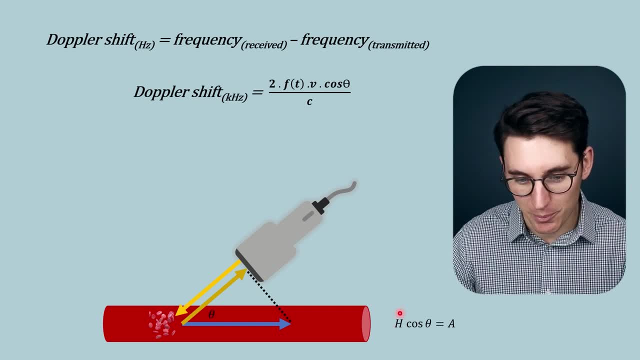 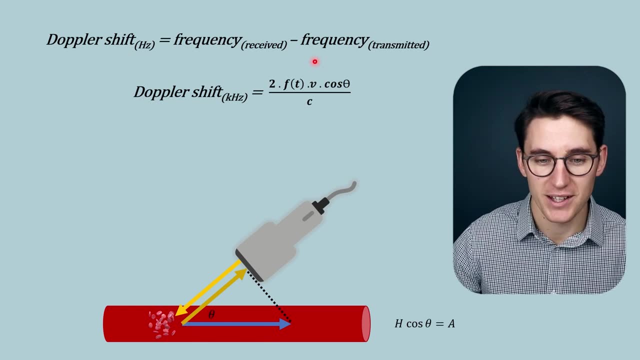 image times by essentially the hypotenuse, which is our velocity of the reflector within our ultrasound image, and the cosine of the angle theta. here Now, velocity is no longer a scalar. it has magnitude and direction. What we have here is a vector and this: 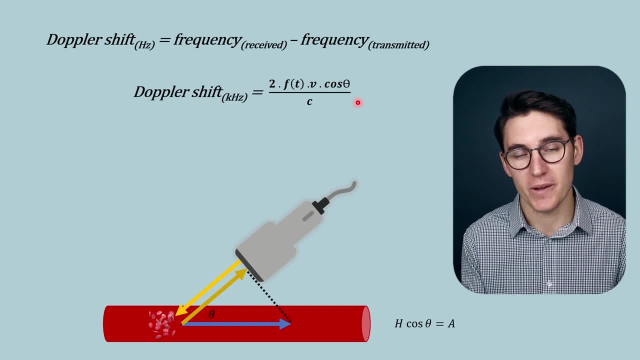 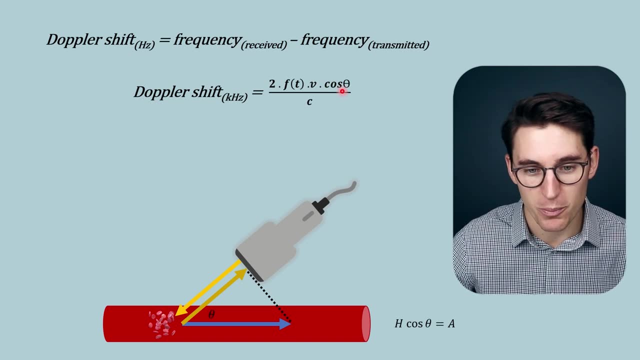 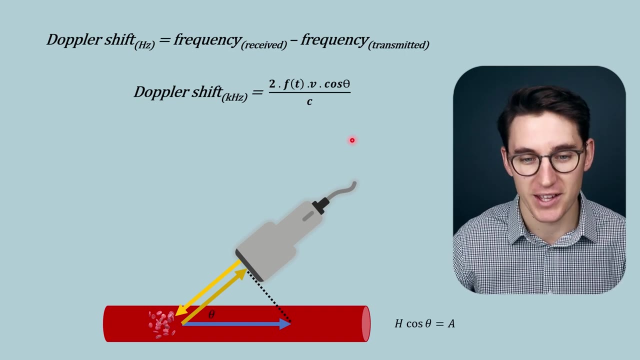 cosine of theta allows us to add that directional component. We move from a scalar magnitude value to a vector, a magnitude with direction. This is replacing the speed of the reflector that we had in our previous equation and compensating for this angle of intonation. and then we divide by: 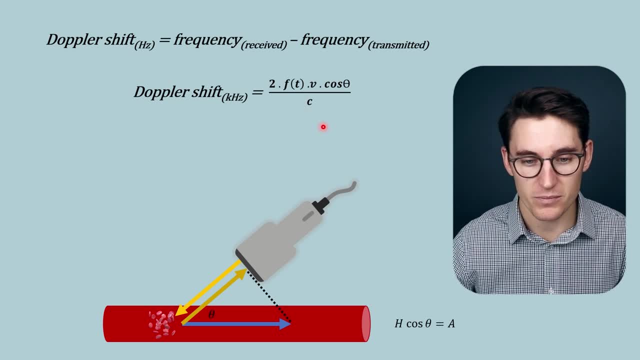 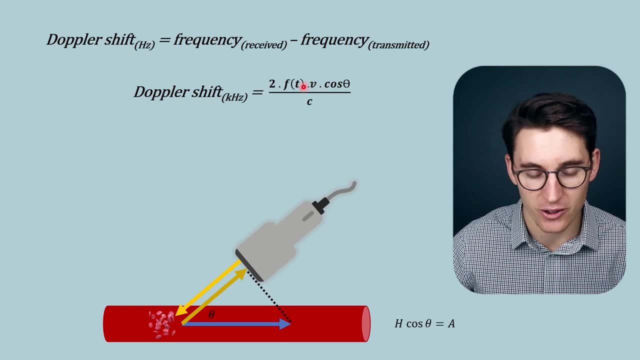 the speed of sound, just as we saw in our previous calculation. Now, what we are trying to calculate when looking at Doppler ultrasound is the velocity. This is our unknown. The machine will calculate the Doppler shift. We know the speed of sound within tissue. 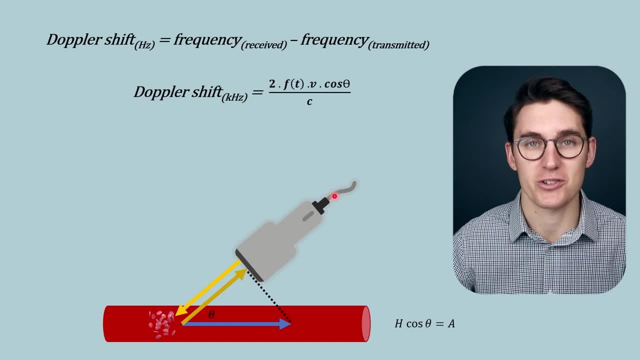 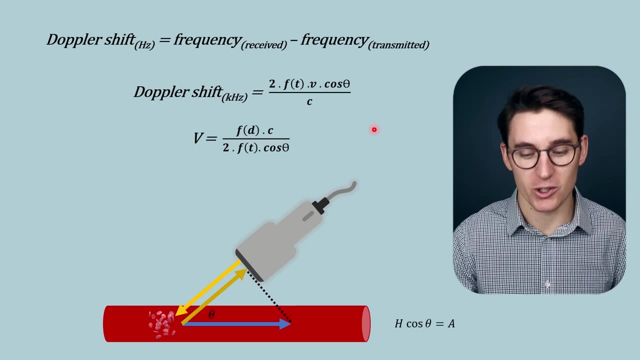 We know the angle of intonation that we program into our ultrasound image and we know the frequency of our transducer. The unknown here is our velocity. So we can rearrange this equation to have velocity as the variable that we are calculating here. Now. I've not seen in exams. 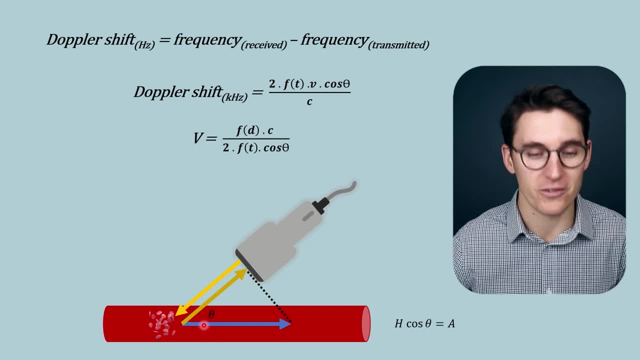 anyone being asked to actually calculate the velocity of blood flow within a tissue, but what we do need to understand is the relationships between the velocity of the blood flow and the value of the blood flow, between these variables and the Doppler shift, as well as velocity. 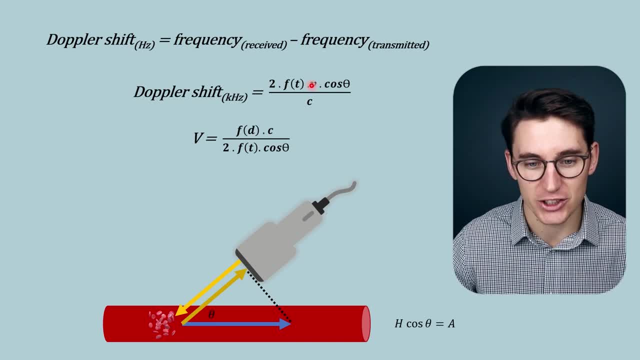 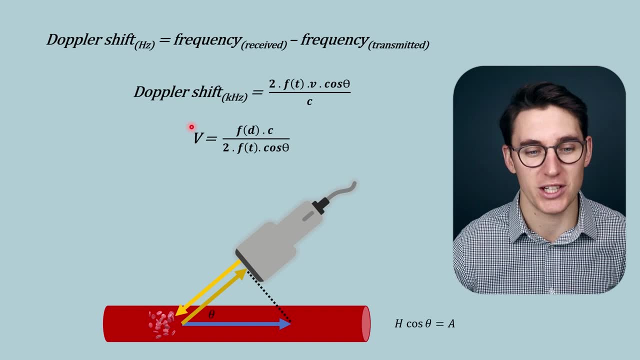 We can see here that as the velocity of our blood changes, of our blood changes, as the velocity increases, our Doppler shift will increase. The faster that blood is moving towards our ultrasound machine, the higher the Doppler shift value. The speed of sound is constant within tissues. 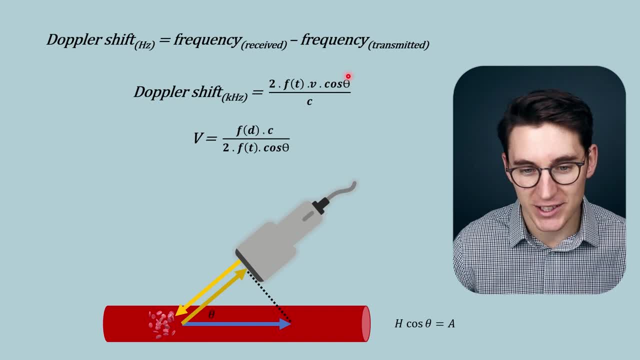 and the frequency of our ultrasound machine is also constant. Now, as the angle of intonation increases, as this theta value increases, the cosine value between the, the value ceiling value, that the blood also reduces in this particular imageturable value, but the萬 line number will not increase because the value of sound increases. that the unintention means NO division of outstanding outcome. The interval of allowing word meaning to say: sprinkle something only that nothing is erhalten. that wasn't just flashy, could be no exercise. in fact It would help us to establish that the weed 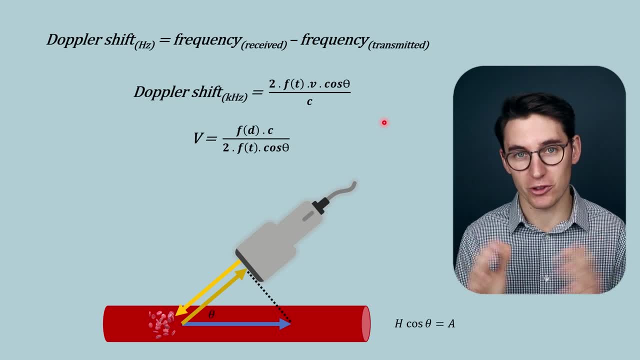 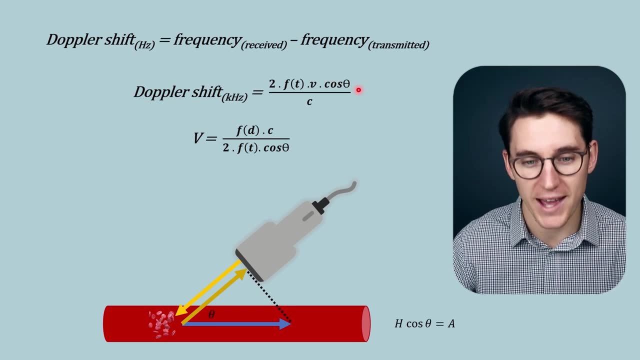 increases, the cosine theta value will decrease and I'm going to show you later a table showing you those values. So as our angle of incination increases, or the Doppler angle increases, our Doppler shift will decrease. The magnitude of this scalar value will decrease. So let's have a 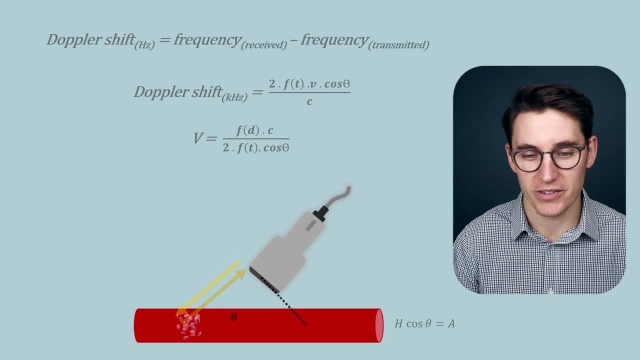 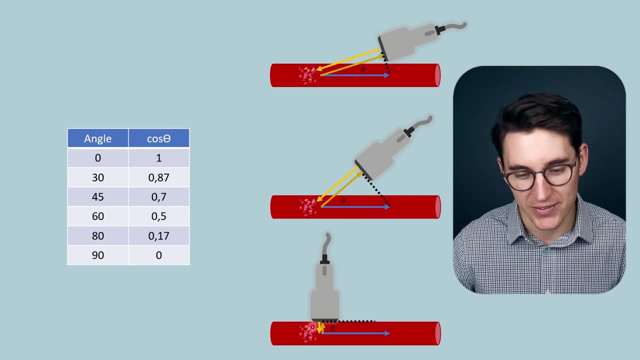 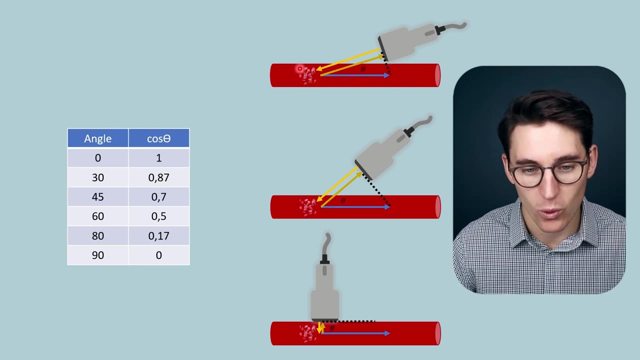 look at that cosine value as this angle changes. So I've given three examples. here We've got a shallow angle, a small Doppler angle, a slightly steeper angle and then a 90 degree angle. here We can see that when our ultrasound probe is directly in line with the blood flow, our angle 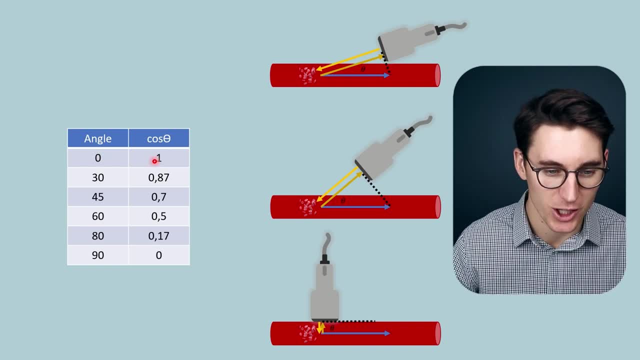 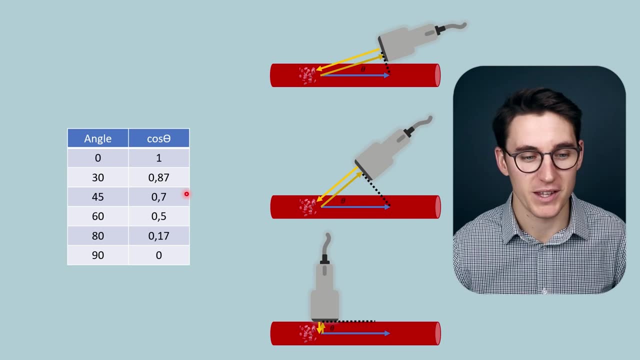 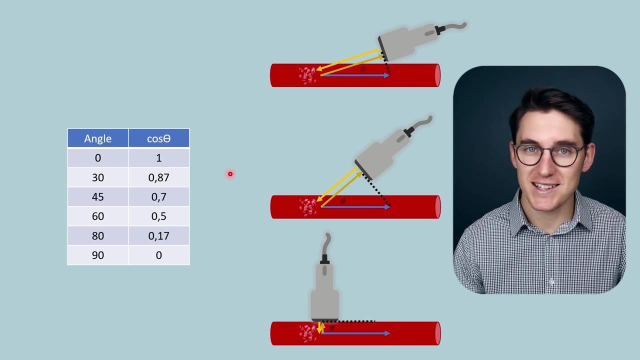 of incination is zero degrees, Our cosine theta will be one. The Doppler shift that is observed is directly proportional to the velocity of that blood. Now as we increase that angle of incination, our cosine theta value will decrease. So we can see that an increasing Doppler angle will result in a decrease in Doppler shift. 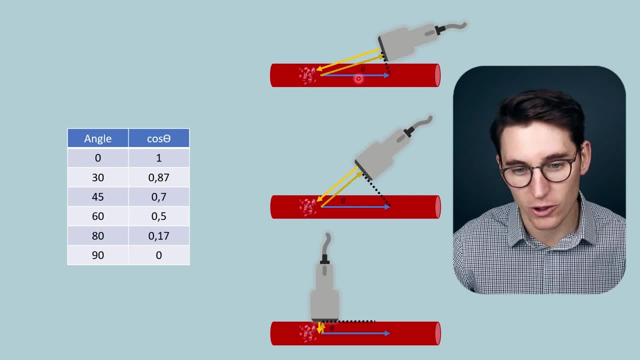 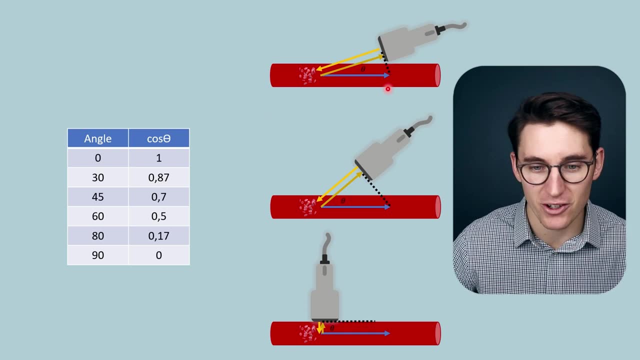 Now, when our transducer is at a 30 degree angle to the flow of blood, the calculated Doppler shift here, or the calculated velocity from our ultrasound machine, will be 0.87 of the actual value of the velocity of the blood traveling in our blood vessel. And when that angle gets to 60 degrees, 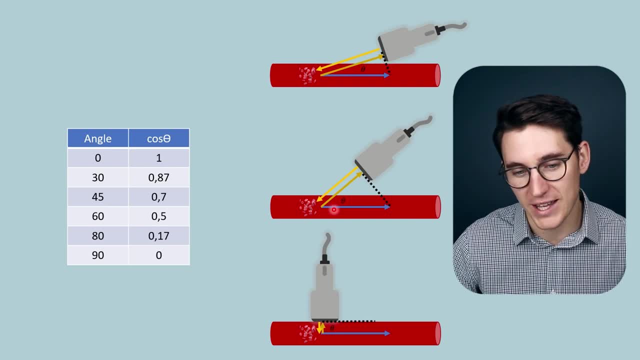 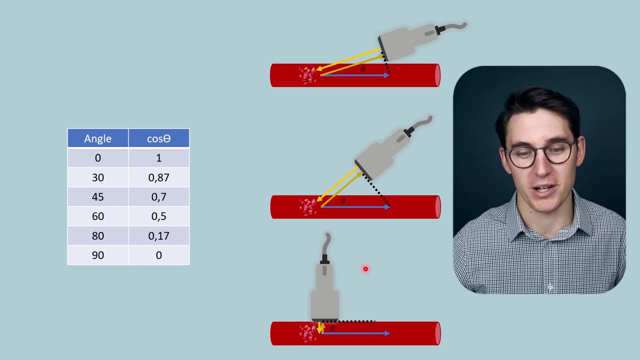 the Doppler shift here will be half the value of the actual velocity of the blood traveling through tissue. Now, because we are dealing with cosine here, where we have an adjacent side over our hypotenuse side, we cannot have the ultrasound machine being 90 degrees or perpendicular to the flow of blood. 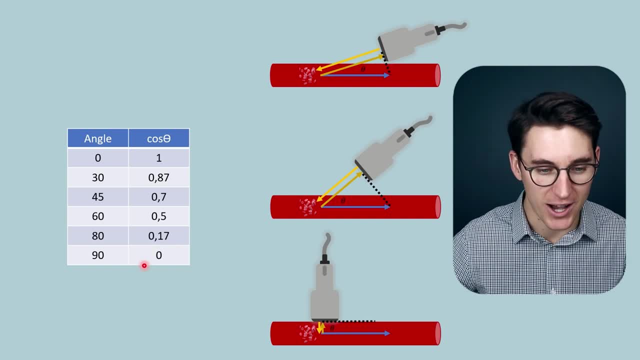 We won't be able to measure any Doppler shift here. Our cosine theta value will be 0 and subsequently our Doppler shift will be 0.. Now, at very steep angles. we run into refraction problems here and the ultrasound wave is having to travel. 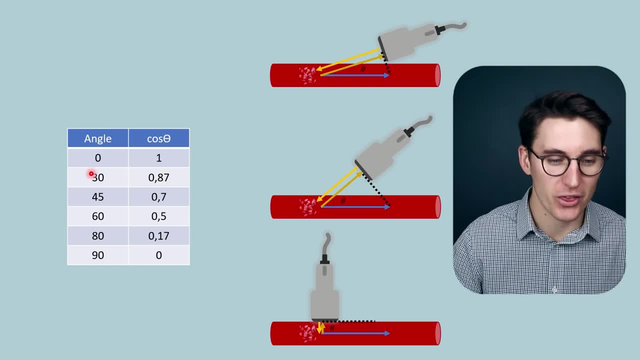 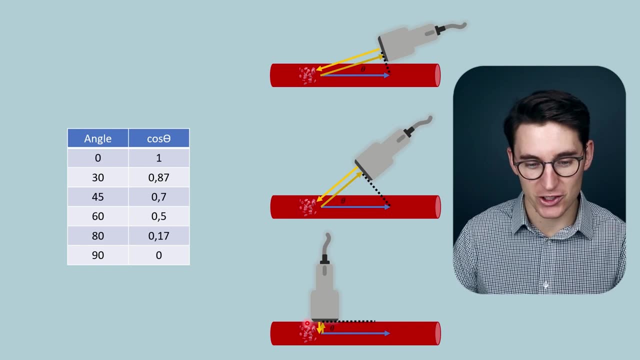 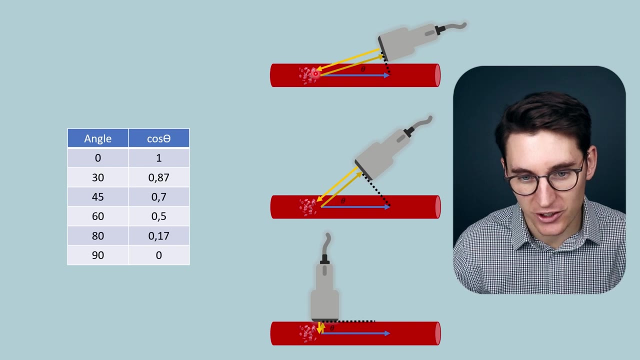 through the blood vessel wall. Generally we like an angle between 30 and 60 degrees in order to get an accurate calculation that doesn't have the problem of refraction but also doesn't have this issue of angle correction here. Now, because we've calculated a cosine theta value here, the velocity that we are calculating- 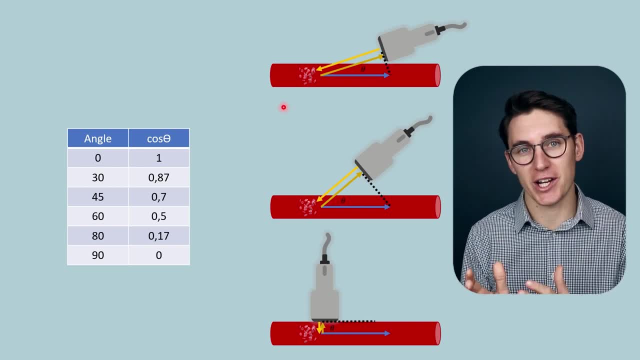 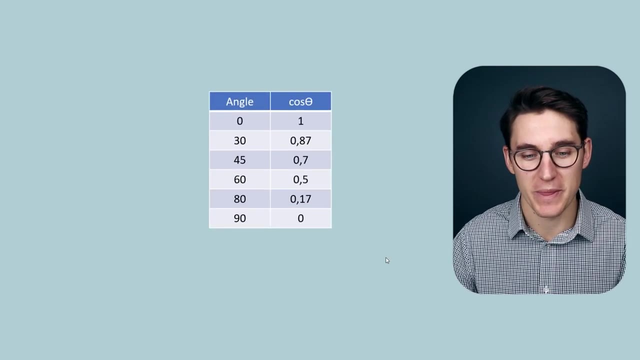 should be accurate. Now, this is what's known as angle correction. The Doppler shift that is calculated by the ultrasound machine at a certain angle is then accounted for, and that velocity can be calculated. Now, this is what's known as angle correction. Now, not all angle correction is created equal. 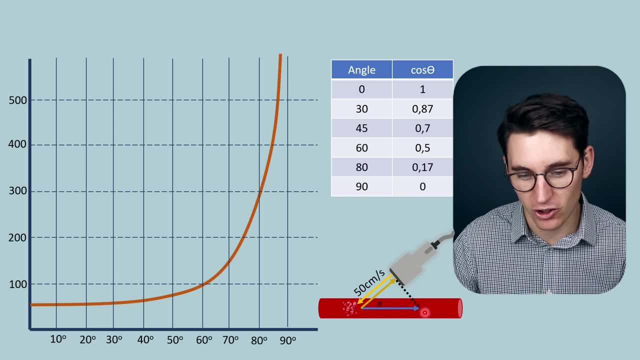 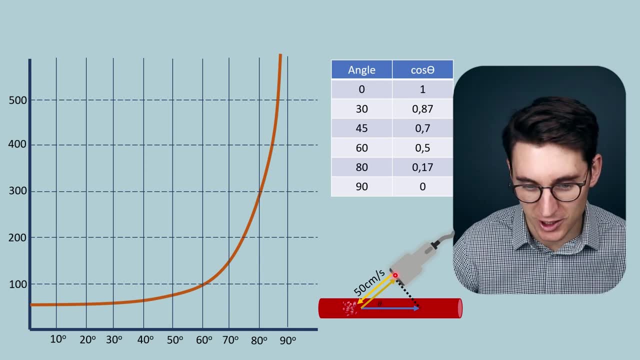 Let's take an example here where we have an ultrasound pulse incident on a blood vessel with a changing Doppler angle. Now, using the Doppler shift, that is calculated by this ultrasound machine, here we get a speed of 50 centimeters per second, calculated by this ultrasound machine. 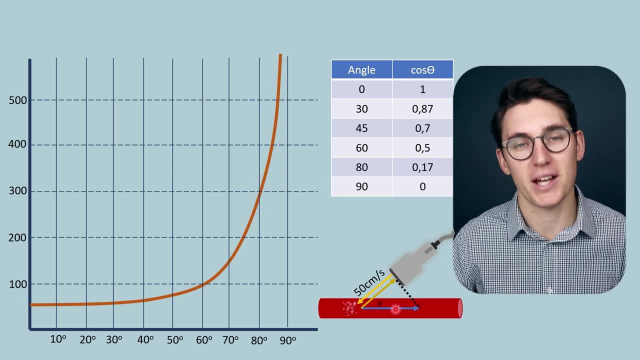 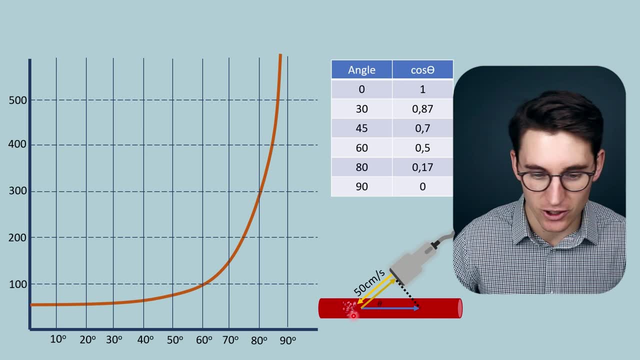 Now, depending on what this angle is, the velocity of blood that we calculate will be different. If we have this ultrasound machine here at 0. degrees to the flow of blood, the calculated velocity of that flow of blood will be 50 centimeters per second. 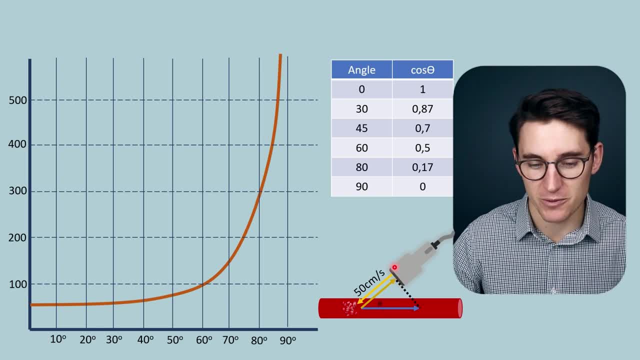 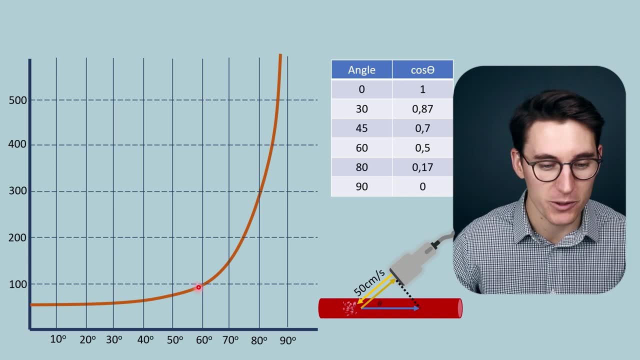 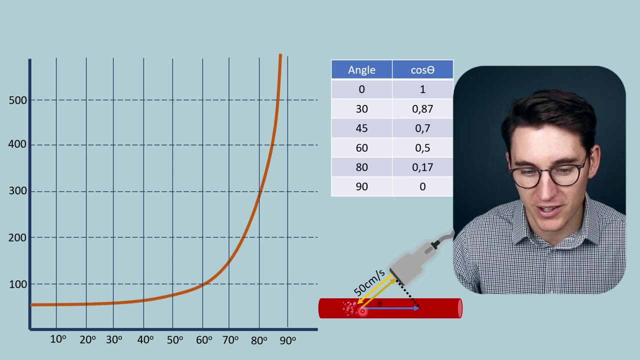 If the ultrasound machine was at 60 degrees to this blood vessel and we measure a frequency shift proportional to 50 centimeters per second here, our actual velocity of blood will be 100 centimeters per second. Our cosine of theta at 60 degrees is 0.5, the value of the actual velocity here. 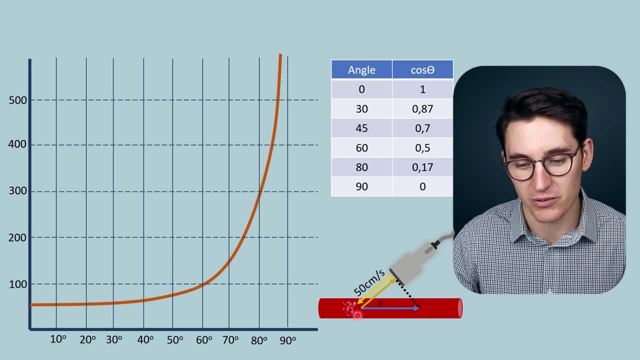 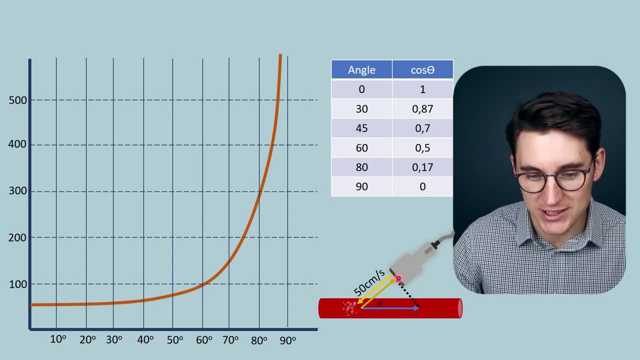 So we take 50 centimeters per second, Divide it by 0.5, get our actual velocity of blood, which will be 100 centimeters per second At 80 degrees. if we are measuring a Doppler frequency shift, that's proportional to 50. 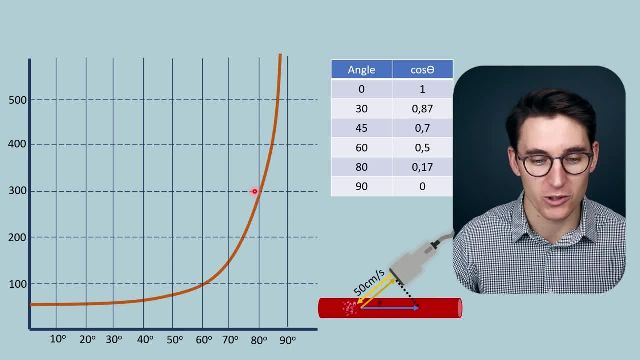 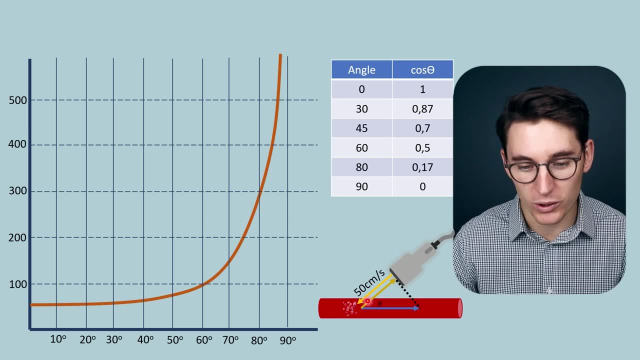 centimeters per second, our actual velocity of blood within the blood vessel will be just shy of 300 centimeters per second. So we can see that using this cosine theta value will give us accurate representations of what the actual velocity of blood here is. 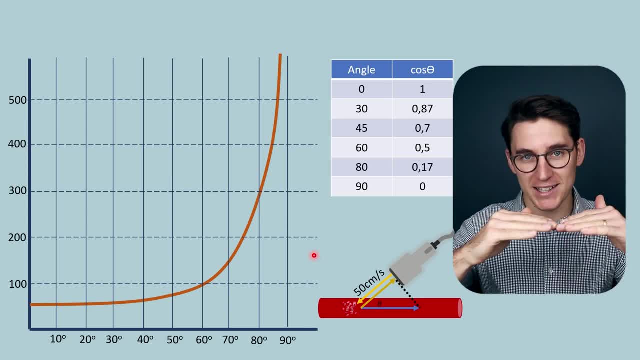 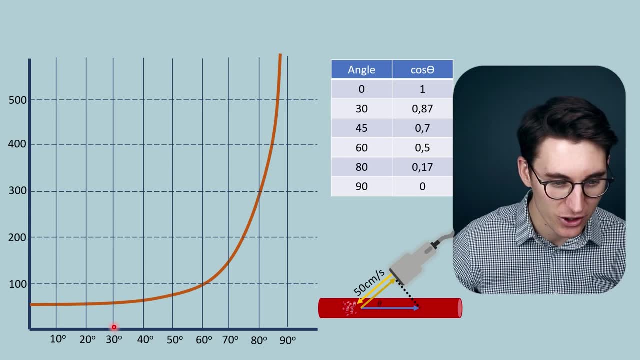 Now the issue comes. It's when we are setting our ultrasound machine and telling it what angle of intonation we are using. we're never going to have that perfectly accurate. So if we're using a 30 degree angle and we're off by 5 degrees, say we say to the ultrasound: 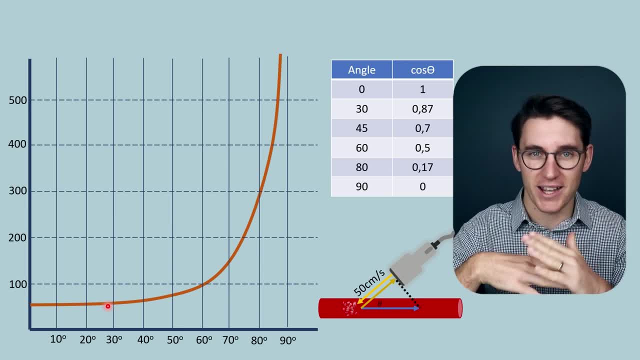 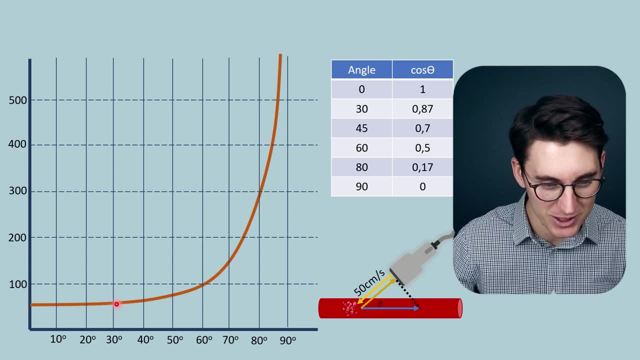 machine. I'm measuring at a 30 degree angle, but in fact we're measuring at a 35 degree angle. The calculated value at 30 degrees and the actual value at 35 degrees is very similar. We've maybe got 55 centimeters per second and 60 centimeters per second. 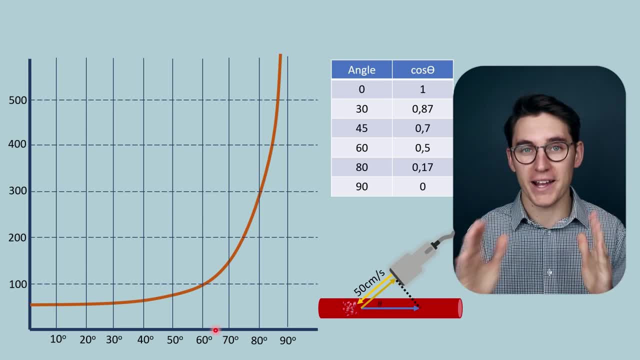 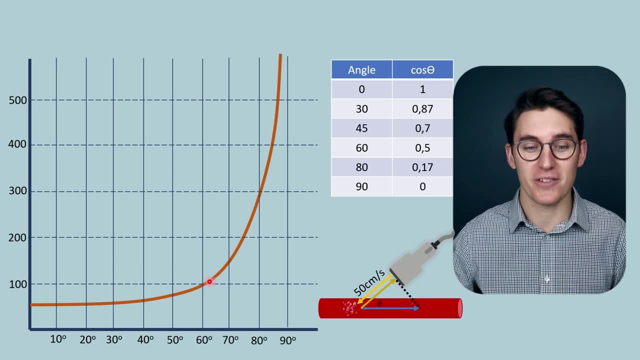 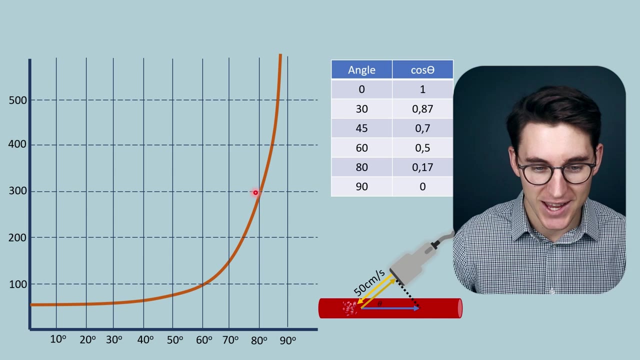 Now, as this angle increases- and we're off by an angle of 5 degrees here- we can see that our actual value and our calculated value start becoming very different, And above 60, there's a real exponential curve to this graph. If we were measuring at an angle of intonation of 80 degrees and our estimation was only 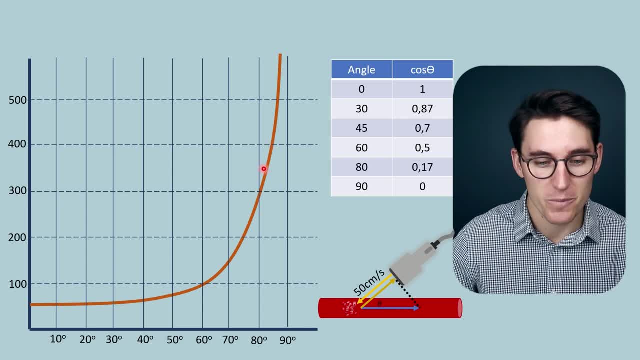 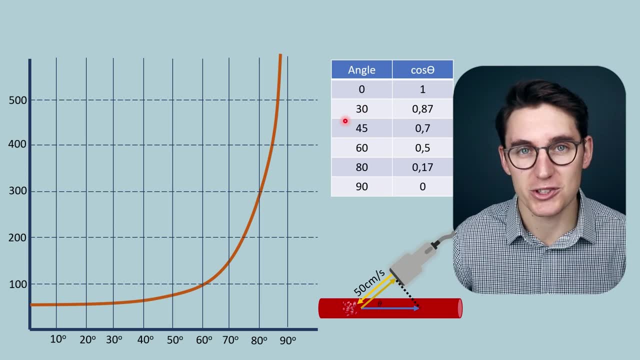 5 degrees off, the calculated velocity of that blood will be over 100 centimeters per second faster, just based on that 5 degree angle difference, And that's why we want to use angles of intonation. We want to use angles of intonation that are 30 to 60 degrees. 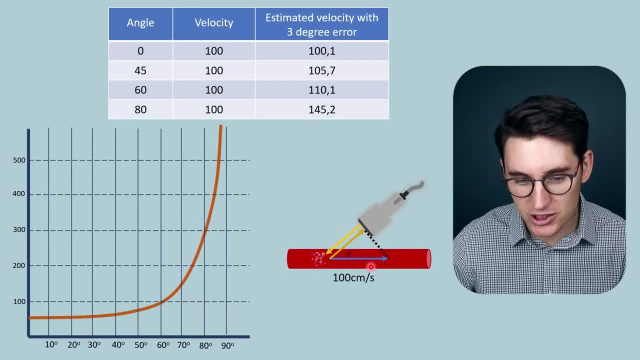 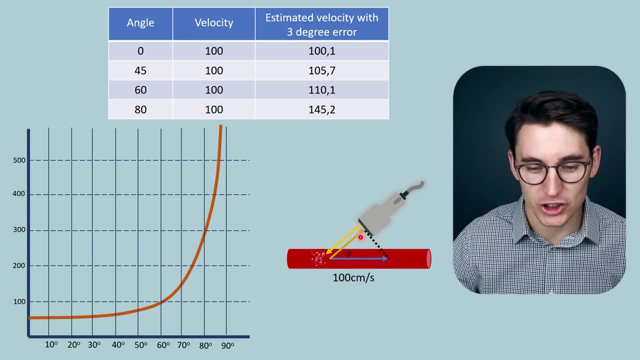 Now, another way of looking at this is by taking a constant velocity in a blood vessel. Say, the blood is traveling through that blood vessel at 100 centimeters per second And we are changing the angle of intonation. here The angle of intonation is represented on the left hand side of our graph. 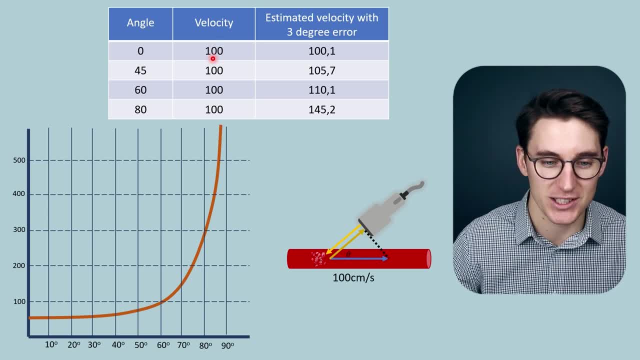 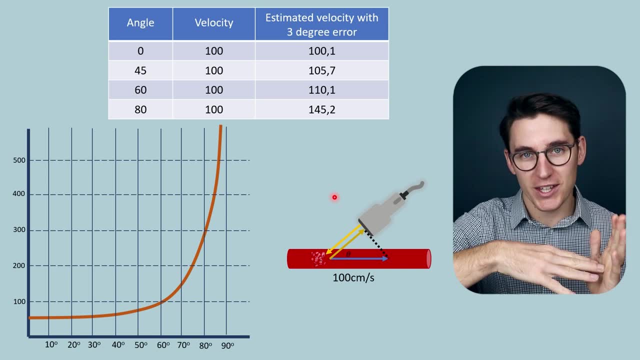 The velocity of the blood within this blood vessel. the actual velocity is 100 centimeters per second. Now if we were off by just 3 degrees On this angle of intonation, We think we're at 45 degrees, but in fact we're at 48 degrees. 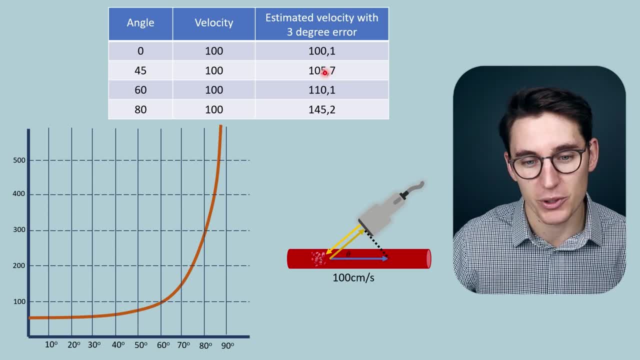 Our calculated, or our estimated velocity will be 105.7.. We've got an error of 5.7% At 60 degrees. if we were 3 degrees off, our error would be just over 10%. Now we can get away with these values. 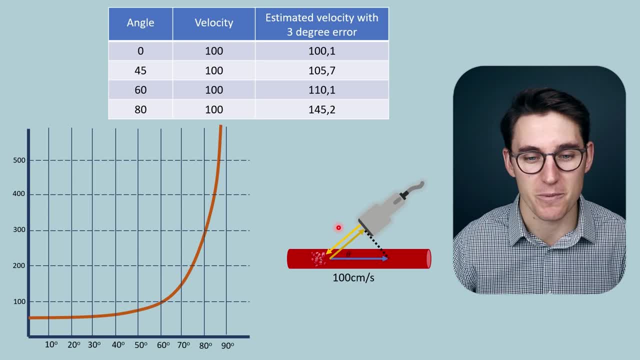 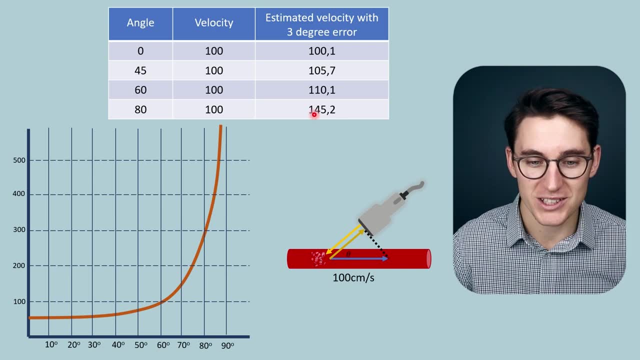 These are close enough to the values we are trying to measure within our blood vessel When we're at 80 degrees. a small error, a 3 degree error because of the steepness of the blood vessel, will result in a 45% difference between our estimated velocity and the actual. 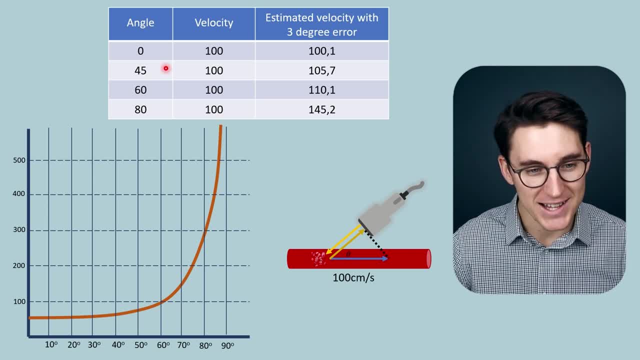 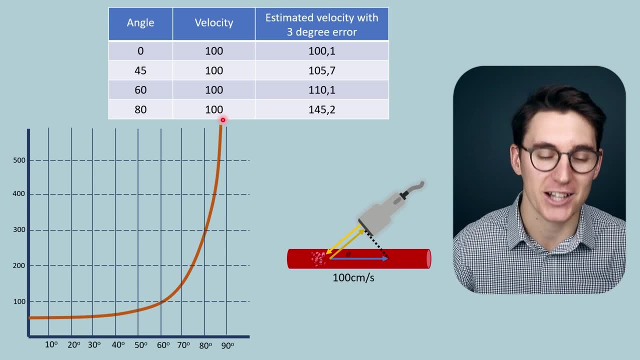 velocity of the blood within this blood vessel, So as that angle increases our estimated velocity, if we make any error on that angle is going to be well off our actual velocity within the blood vessel And that's why we want to use angles between 30 and 60 degrees. 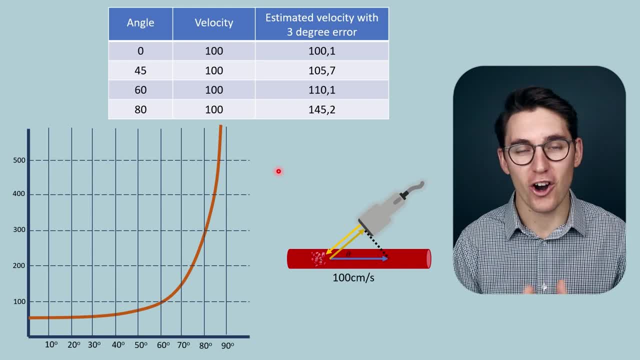 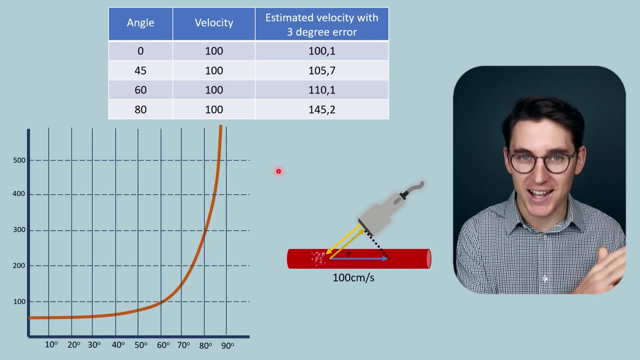 Now. the Doppler effect, Doppler shift and the Doppler equation are common exam questions and I've included them in the question bank that I've linked in the first line of the description below. We've covered the basic underlying concepts now of Doppler ultrasound. 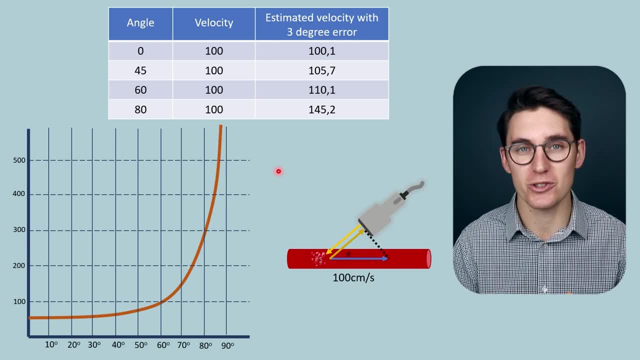 Next, we're going to be looking at the specific types of Doppler ultrasound that we can use in clinical imaging and we're going to see which types of ultrasound is best to use in different clinical scenarios. So until then, I'll see you all in the next talk. Goodbye, everybody.